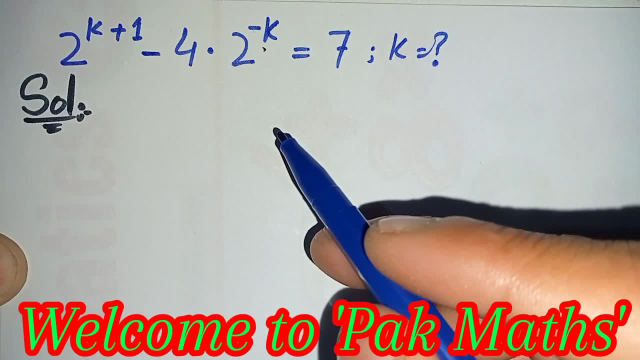 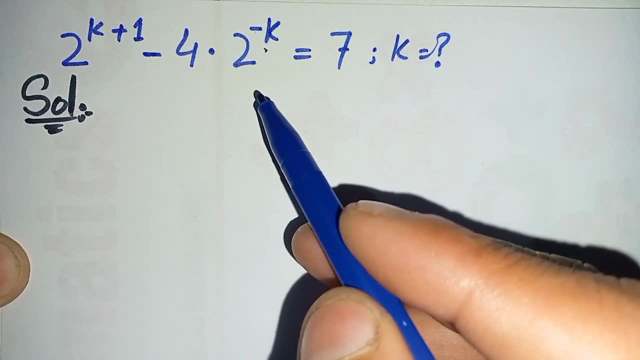 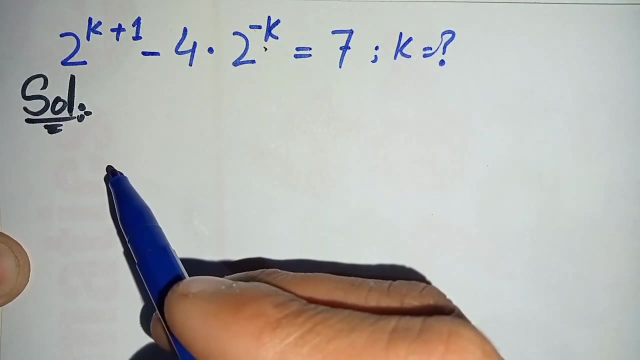 hi everyone, welcome to park maths in this video. I'm going to solve this nice exponential equation. now, to solve this nice exponential equation properly and step by step, first we will write solution and then we will write this question in the solution again. we will try to solve it step by step. the 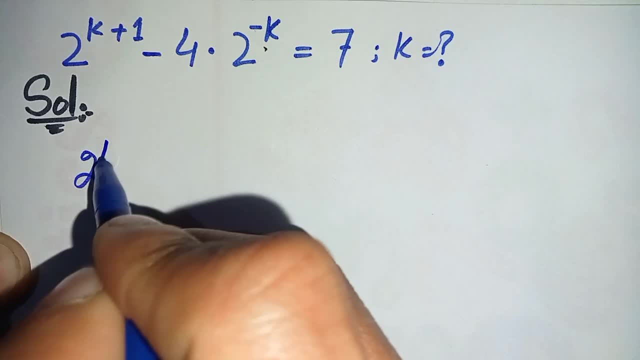 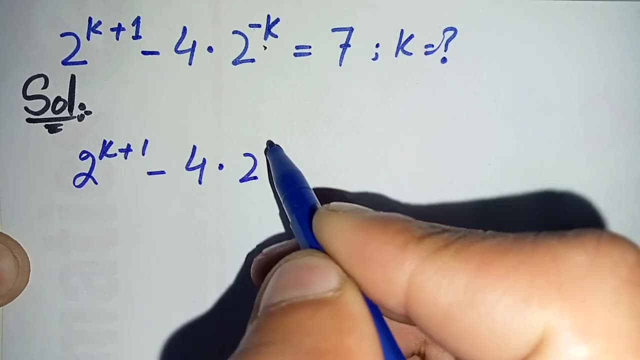 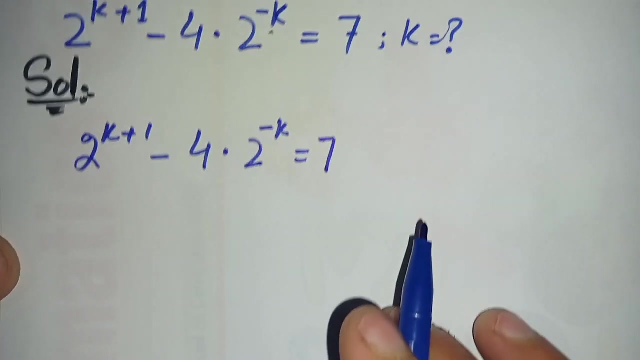 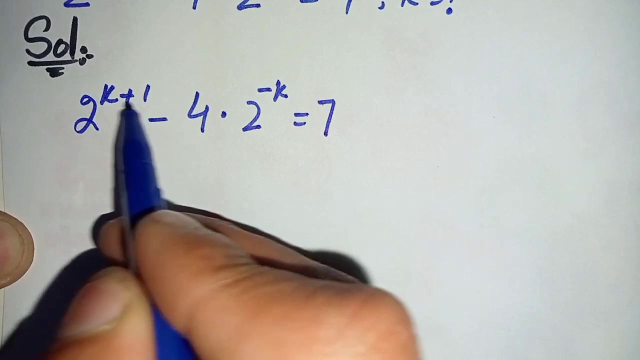 question is: 2 raised to power, k plus 1 minus 4 times 2 raised to power minus k is equal to 7. here, in this term of the equation, we will use an exponential math property and we will split these two terms in the power over the base. so here: 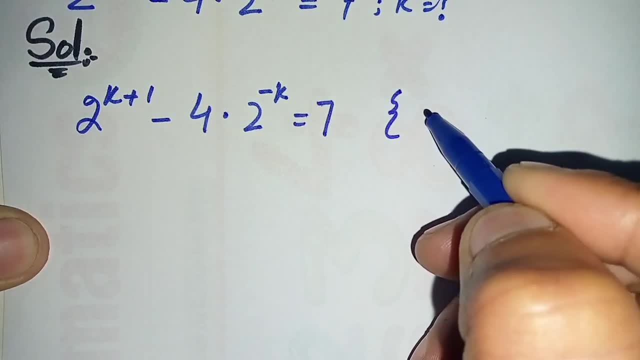 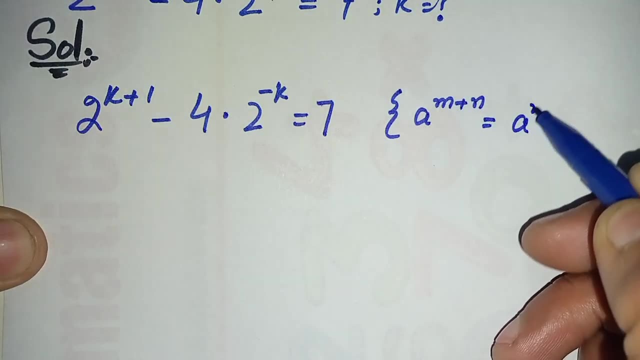 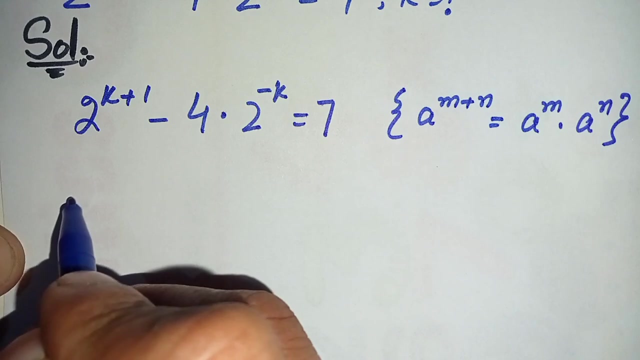 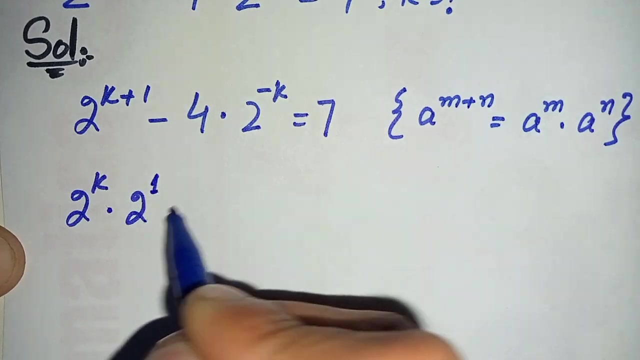 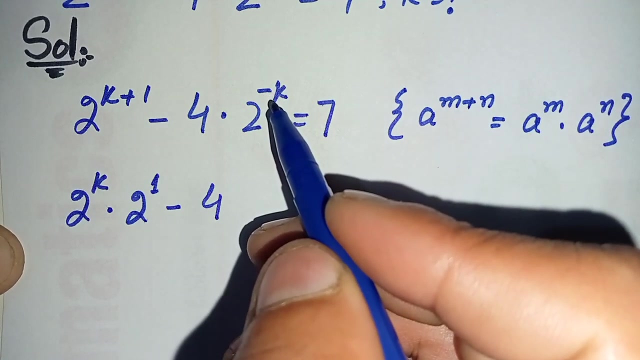 we will use this exponential math property. a raised to power m plus m can also be written as a raised to power m times a raised to power n, so this will become 2 raised to power k times 2 raised to power 1 minus 4. now here we will try to make this power positive, but 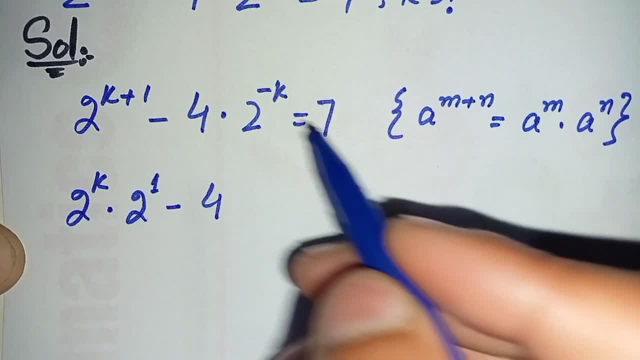 here we will try to make this power positive. but here we will try to make this power positive. but to make this power positive, we will shift this to make this power positive. we will shift this to make this power positive. we will shift this whole number to the denominator and. 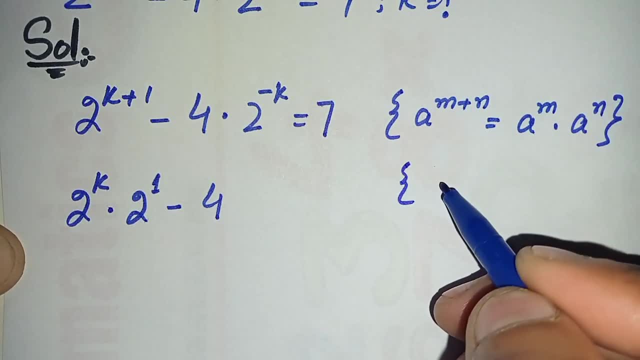 whole number to the denominator and whole number to the denominator. and here we will use this exponential math. here we will use this exponential math. here we will use this exponential math. property a raised to power minus n. can property a raised to power minus n. can property a raised to power minus n can also be written as 1 over a raised to. 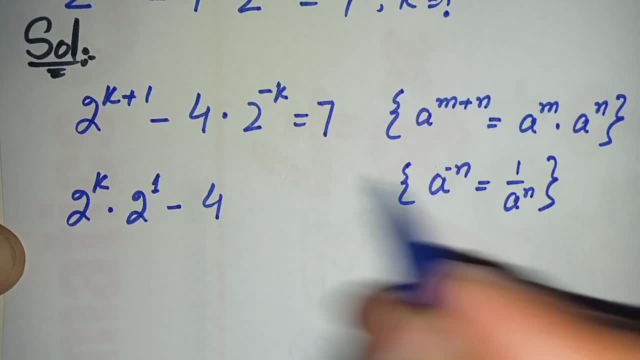 also be written as 1 over a raised. to also be written as 1 over a raised to power n. so using this property in this power n. so using this property in this power n. so using this property in this term, it will become times 1 by 2 raised. 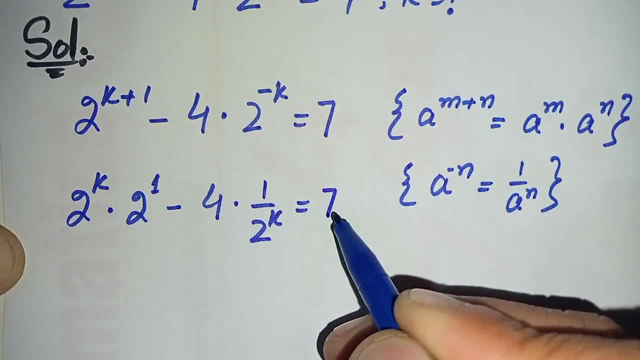 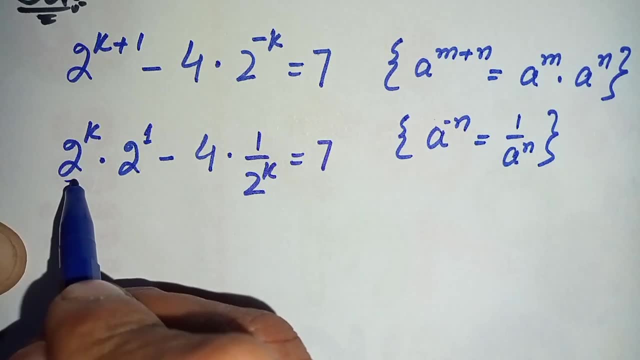 term: it will become times 1 by 2. raised term: it will become times 1 by 2 raised to power. k is equal to 7. now, my dear's, look it. to the left hand side of this equation, there's 2 raised to power k. 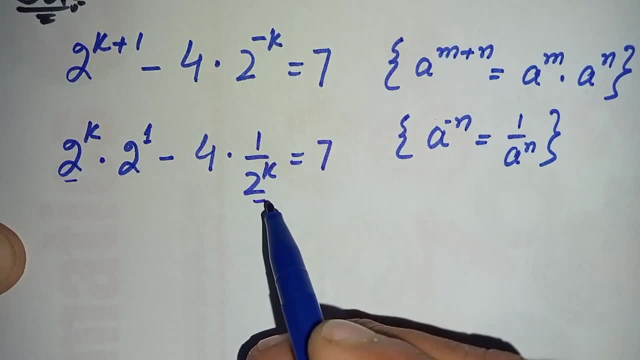 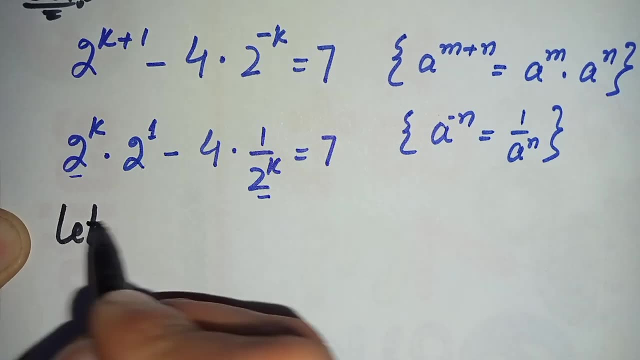 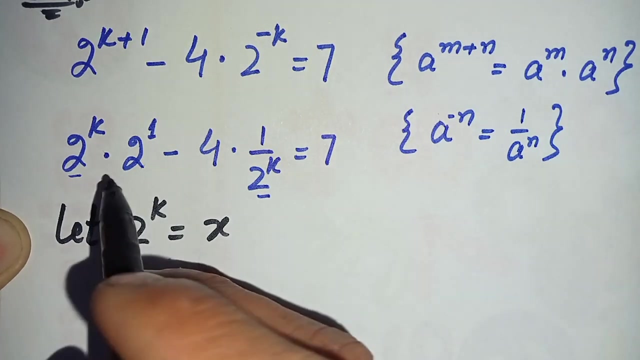 there is also 2 raised to power k in the denominator, so here we will make a supposition. so let us suppose let this 2 raised to power k is equal to X. so here we will replace 2 raised to power k in this equation with X. so this equation: 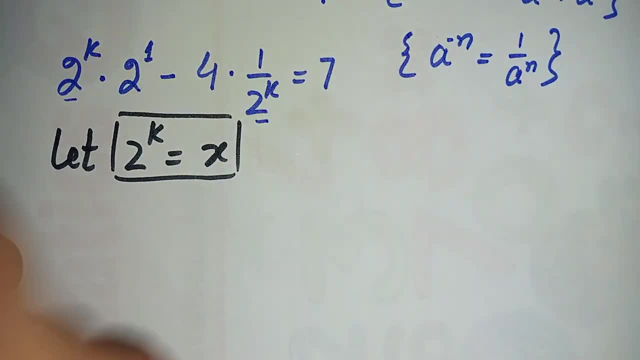 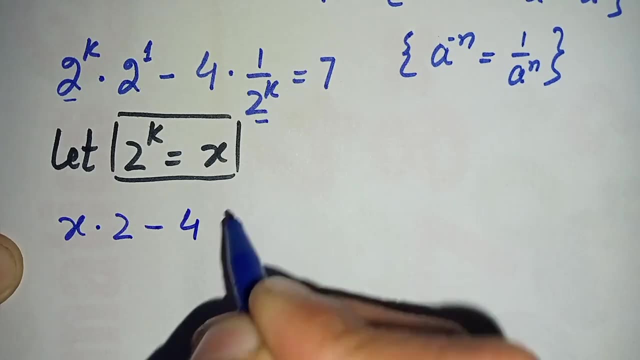 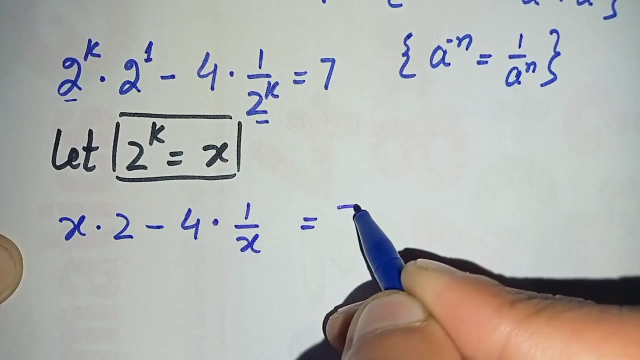 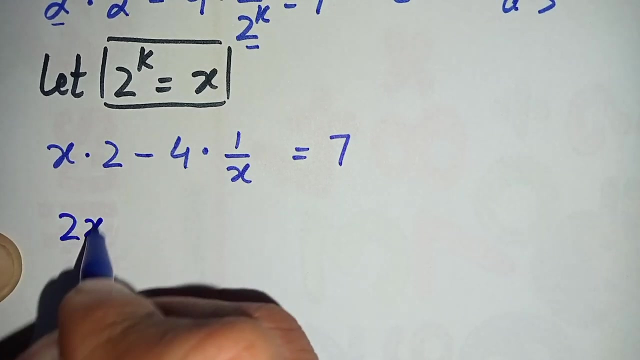 will become? will become X times 2 raised to power. 1 is equal to 2 minus 4 times 1 by X is equal to 7. now further, let's simplify this equation, so it will become 2 X minus 4 times 1 over X. 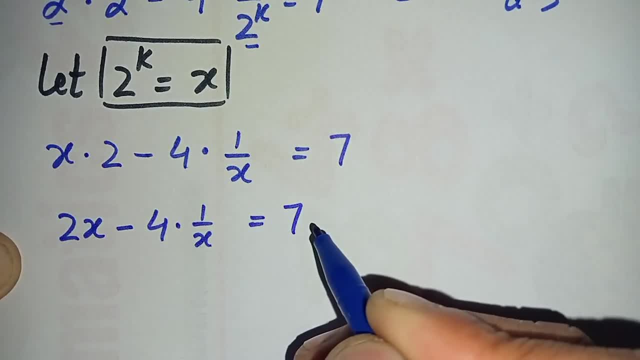 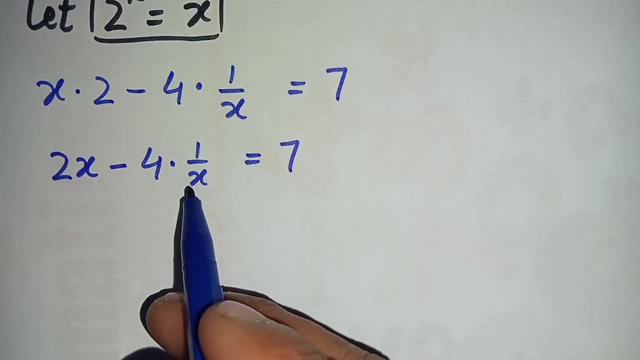 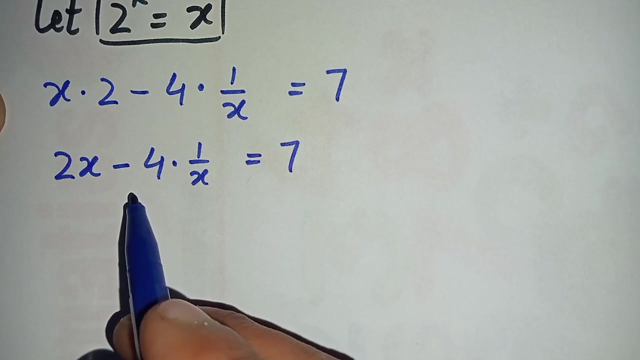 is equal to 7. now, here we will try to eliminate this X from the denominator. now, to eliminate this X from the denominator, there are two approaches to eliminate it. one is to take a seam of these two terms, and the second step is: and the second approach is to multiply X in both sides of this equation. so let's 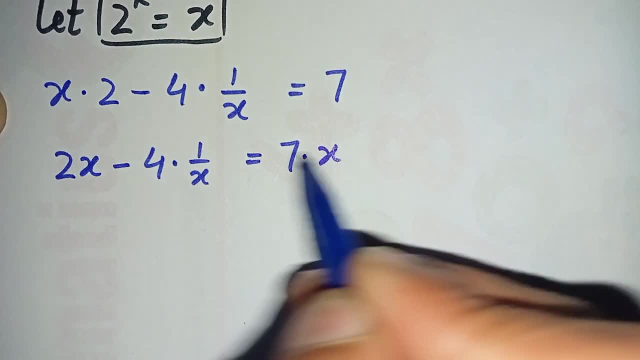 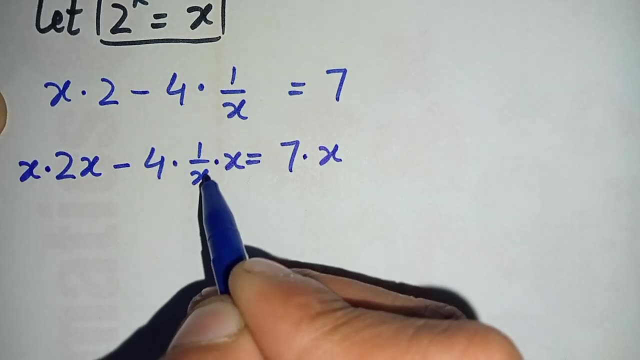 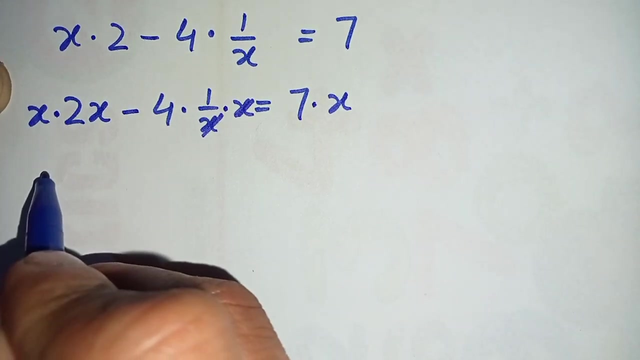 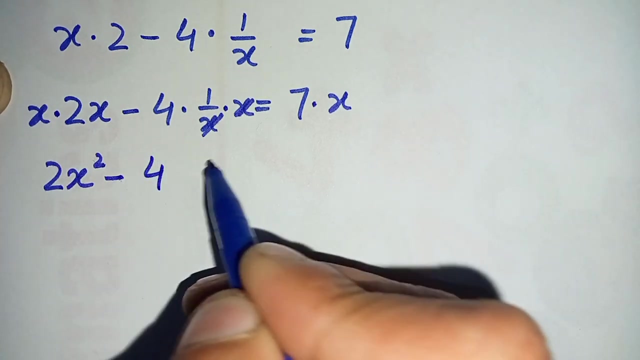 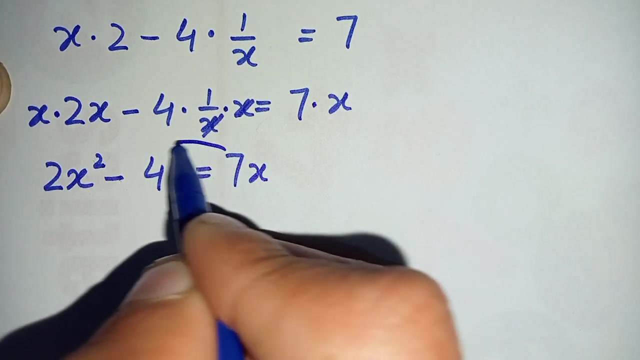 multiply X in both sides of this equation. so it will become: we will multiply X with both the terms here. so here this X and this X will be cancelled with each other, and here we will multiply this X with this, so it will become minus. here only power, as let is equal to 7 X. now, here we will shift this 7 X to. 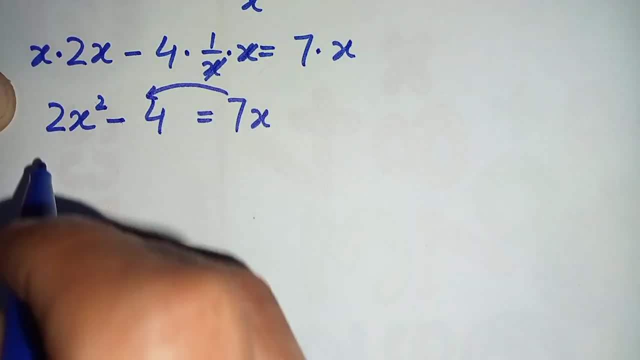 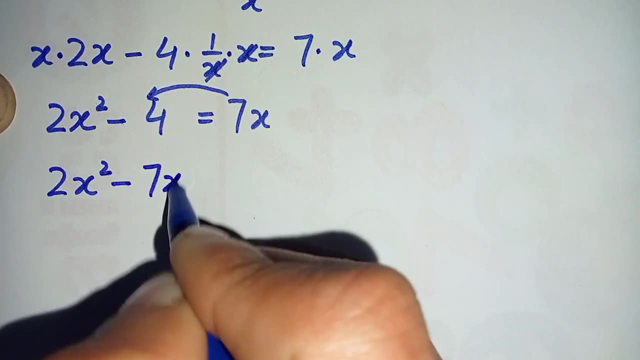 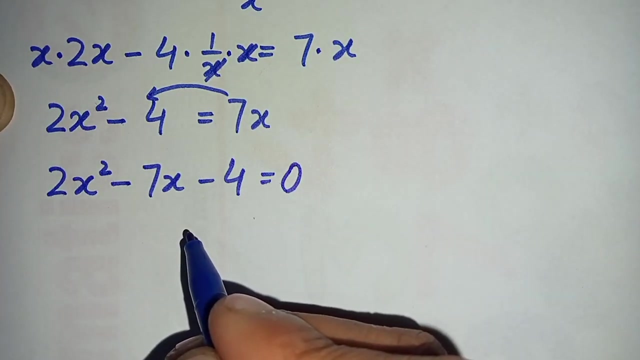 the left hand side. so it will become X square, it will become minus 7. X minus 4 is equal to 0. now this is a quadratic equation. so here we will solve this quadratic equation by factorization method. so to solve it by factorization method, we will find such two numbers: 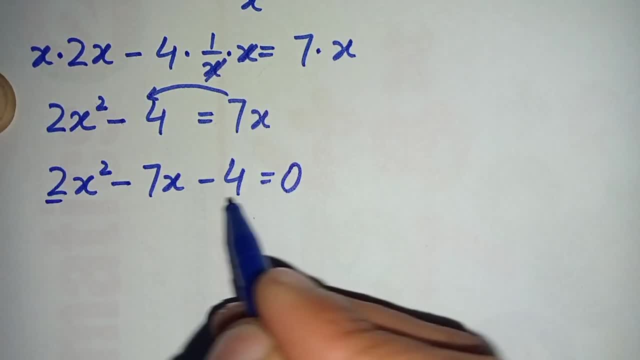 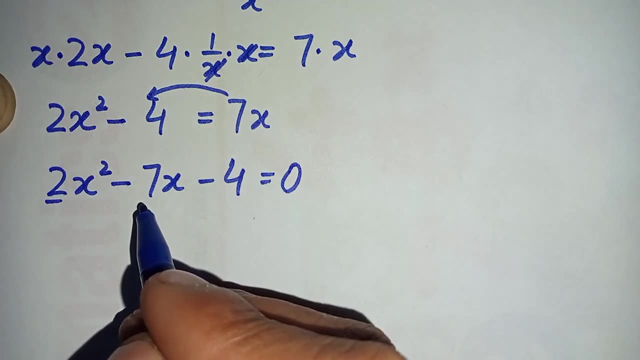 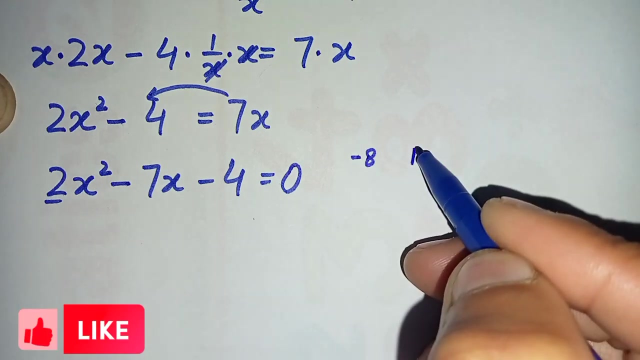 whose product is equal to the product of 2 and minus 4, so the product of 2 and minus 4.. 4 is minus 8 and their sum is minus 7. so these two possible numbers may be minus 8 and plus 1, because if you multiply these two numbers we will get minus 8. 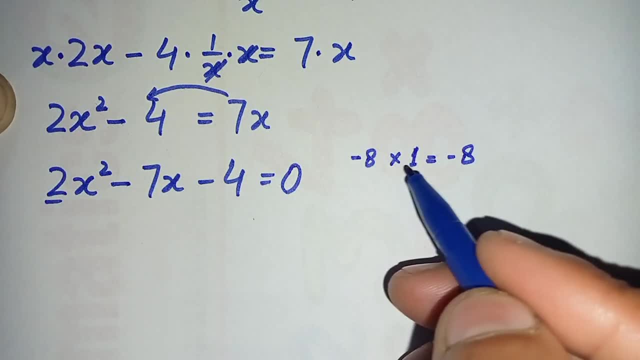 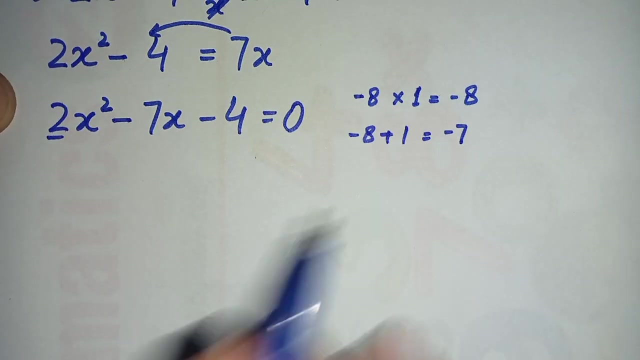 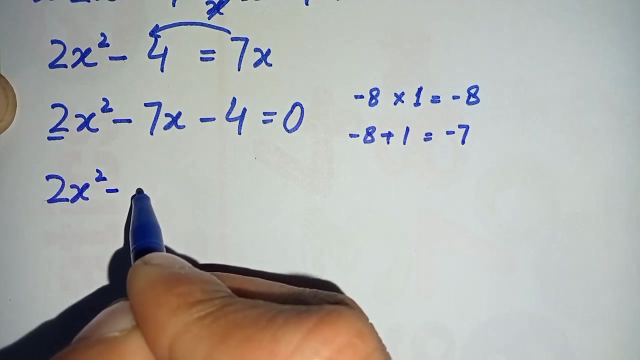 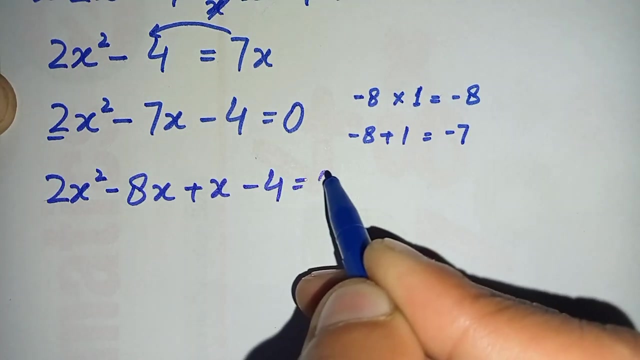 the product of 2 and minus 4, and if we add these two numbers, so we will get this one number minus 7. so here we will replace minus 7 X with minus 8 X and plus X, so this equation will become two times x. square will become minus 8 X plus X. minus per is equal to 0. now here 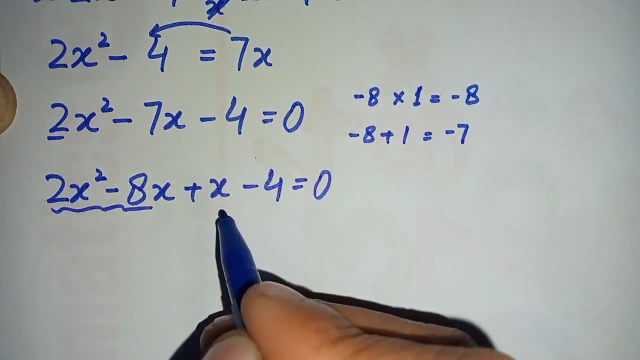 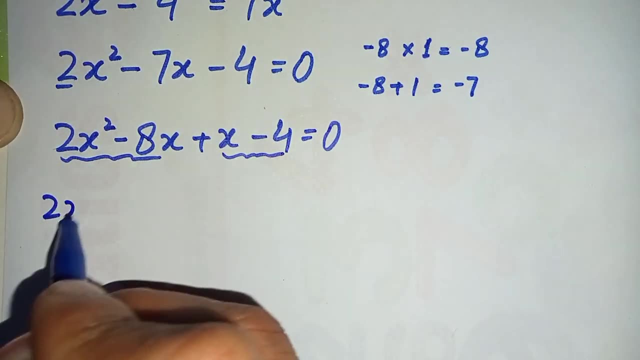 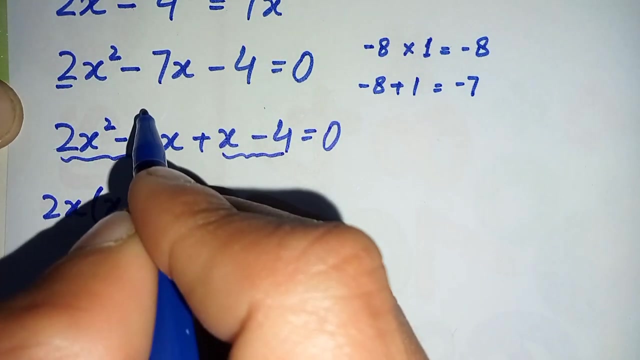 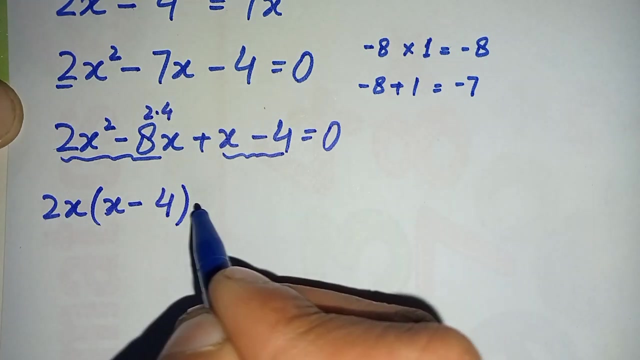 from these two terms we will take 2x common. and from these two terms we will take one common. so it will become: it is take 2x common. from these two terms here only x is left minus. here it can be written as two times four. so two are taken common. so here only four is left plus. from here we will take 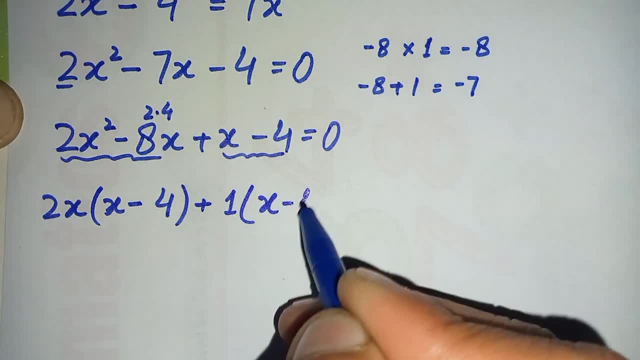 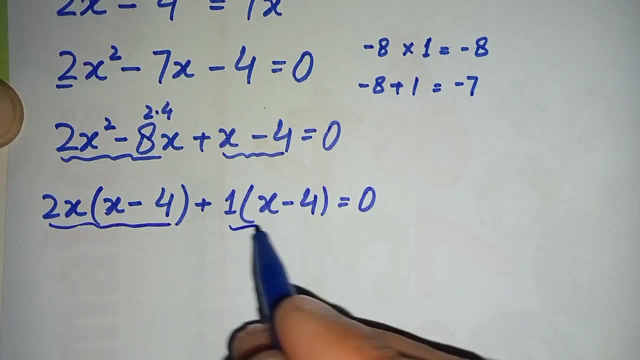 one common, so it will become x minus four is equal to zero. now from these two terms we will take x minus four common, so it will become taking x minus four common. here two times x is left plus, and here only one is left, is equal to zero. 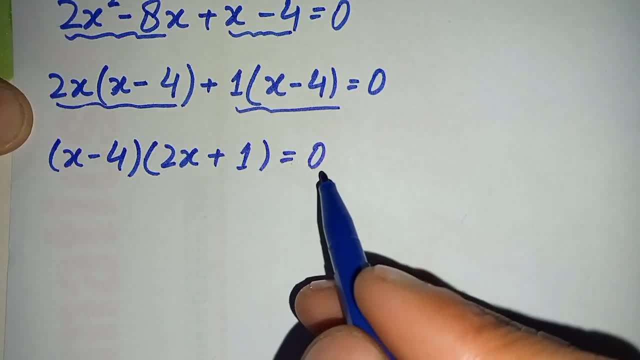 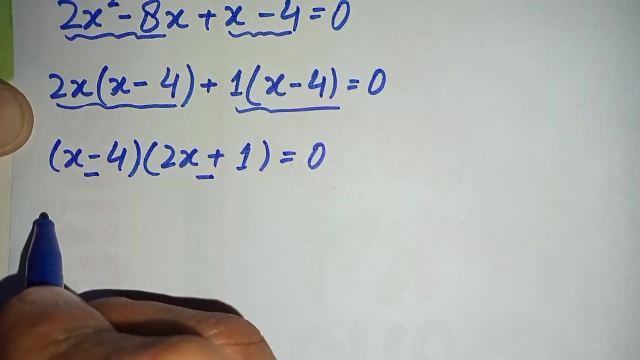 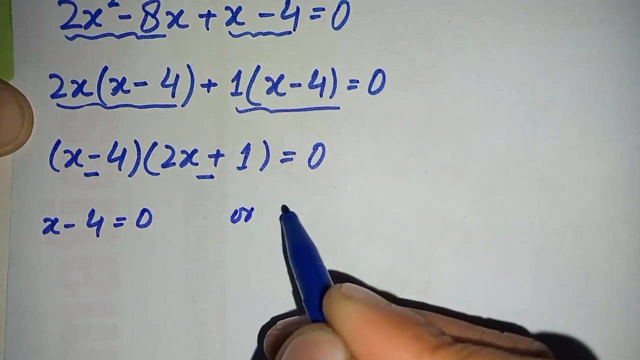 now my dears. here the product of these two expression is equal to zero. so here, either this expression will be zero or this expression will be zero. so we can write them as here: x minus 4 will be 0, or 2x plus 1 will be 0. 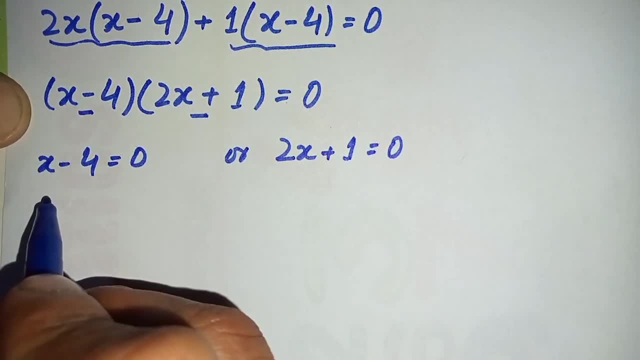 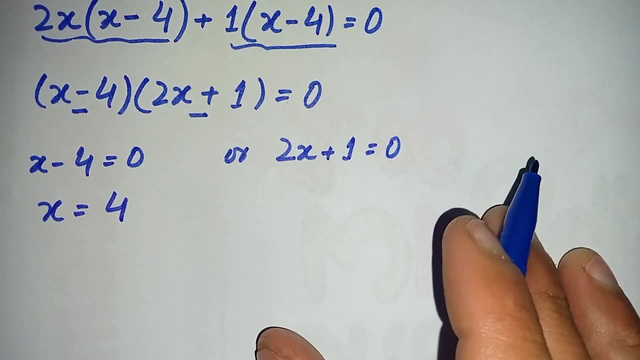 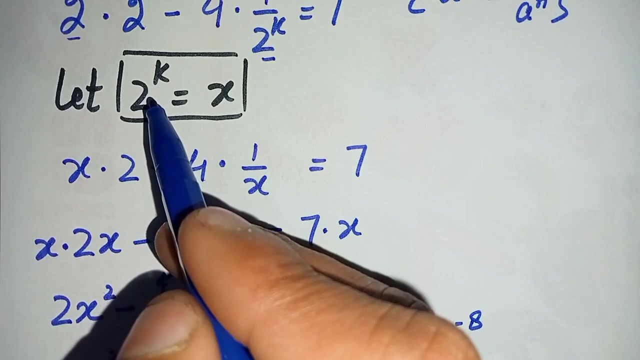 now. first we will solve this one equation. so we will shift this minus 4 to the right hand side, so it will become plus, this requirement, and we will show that heart value is equal to three times 4. but here we need not to find the value of x, here we need to find the value of k from our supposition. 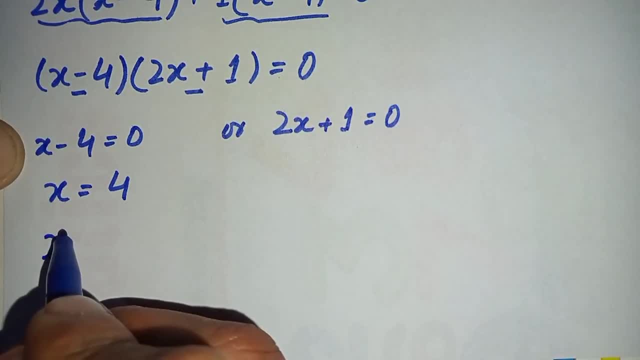 so here we will replace x with 2 to power k. so this equation will become: we will replace x with 2 raised to power. k is equal to power, but we can write to get to both sides. in both sides the bases are same two. so here we will compare the powers with. 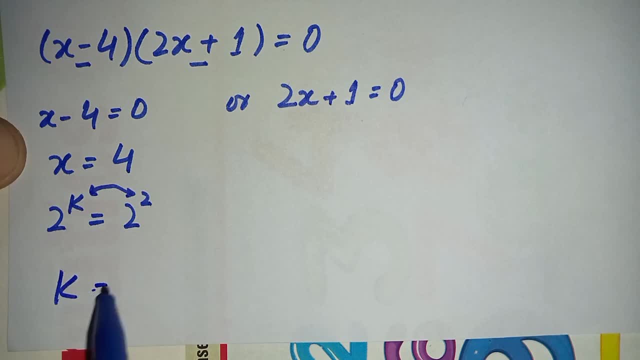 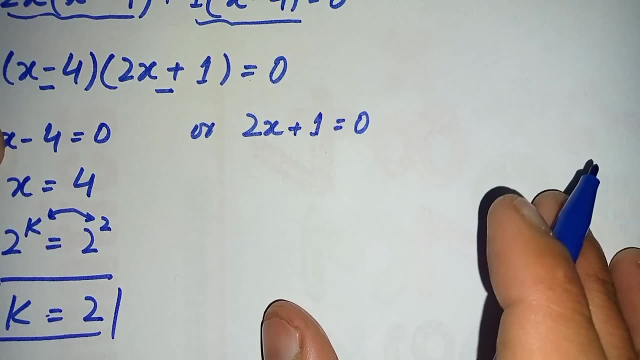 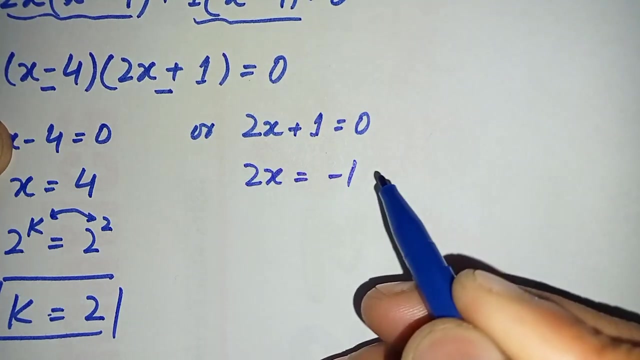 each other. so the powers are k is equal to two, so k is equal to two, is one of our possible solution. now we will try to solve this one equation. so here we will shift this one to the right hand side, so it will become minus one. now we will divide both sides by two, so this two and this. 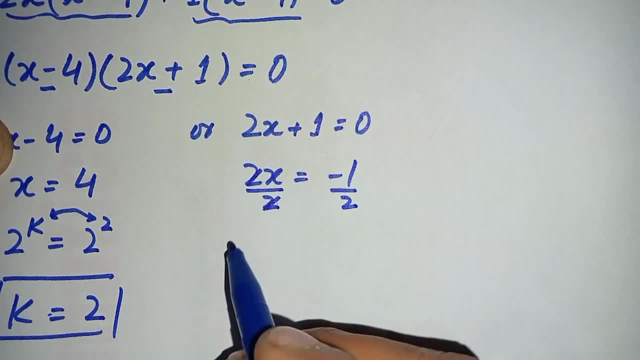 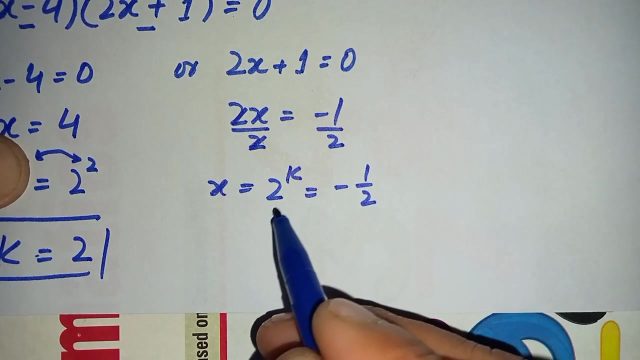 two will be canceled with each other, so only x will be left, and here we will replace this x with two raised to power k. two raised to power k is equal to minus one by two. now, my dears, look into this equation: two raised to power k is equal to minus one by two. 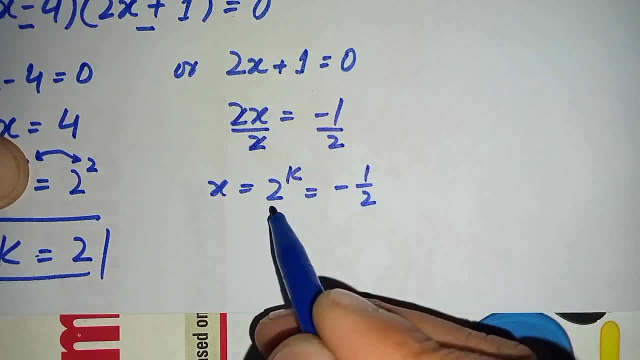 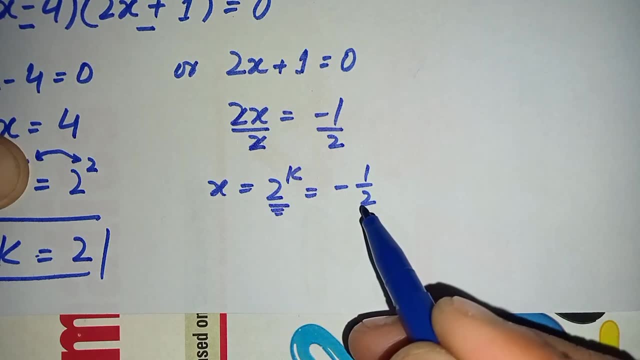 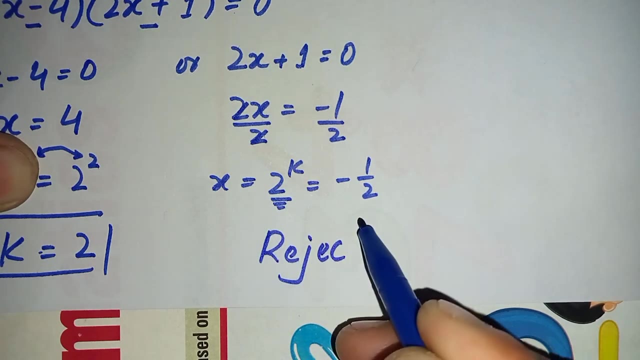 here for any value of k two raised to power, k is always positive, but this is a negative number. so a positive number cannot be changed, not be equal to a negative number, so so that's why here we will reject this one solution. so finally, k is equal to two is one of the possible solution of: 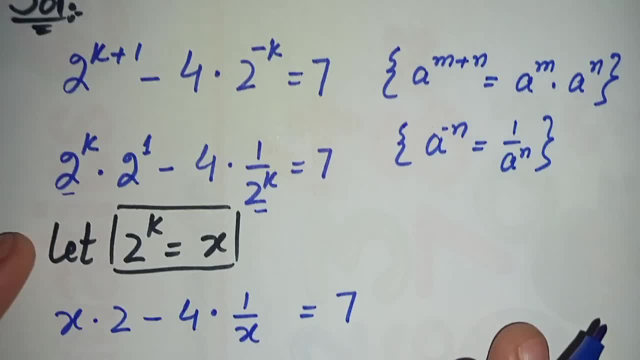 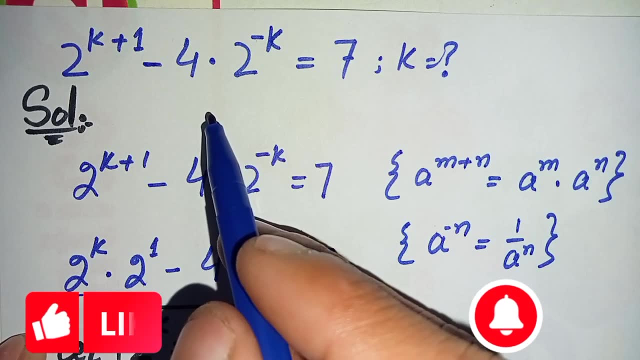 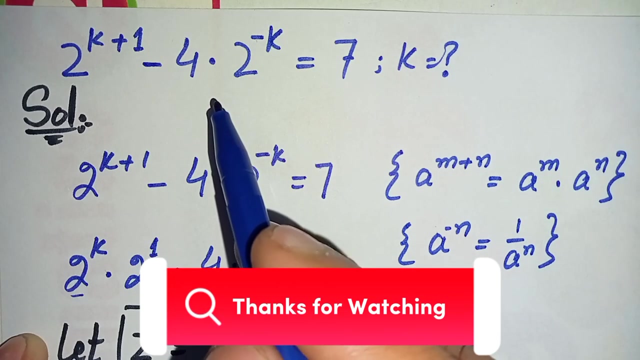 this interesting exponential equation. and last, don't forget to subscribe our youtube channel for such a more interesting math videos. thank you so much for watching. take care, see you in the next video. bye, bye.